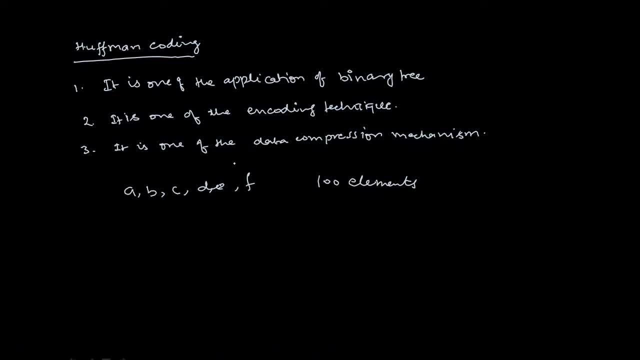 Hello guys. so in this video we will continue our chapter on greedy algorithms. So this is another problem which is solved by greedy technique. So this is also greedy algo. So we solve this halfman coding problem by greedy algo. So what is the halfman coding problem? It is one of the application of binary tree, It is one of the encoding technique and it is one of the data compression mechanism. What actually can be understand by the halfman coding is if we have set of symbols, given like A, B, C, D, E, F, and there is a message in which there are 100 elements. 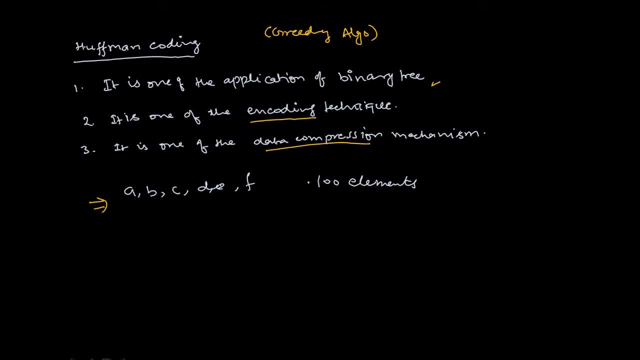 Those 100 elements are only take these symbols. So it may possible that some of the symbols are repeated in order to form a word or a message. So suppose the symbol A is repeated 50 times in the message and B is repeated 2 times and C is repeated 8 times and D is repeated 30 times and E is repeated 6 times, and suppose F is repeated 7 times. 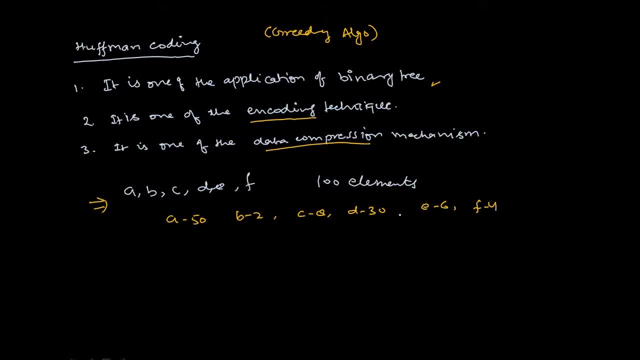 So these are the repetitions of symbols. To send the message to the receiver, we need to convert this message into some encoding set. Generally, if we consider ASCII encoding set, then it will take 7 or 8 bit to encode one symbol and there are 100 elements. 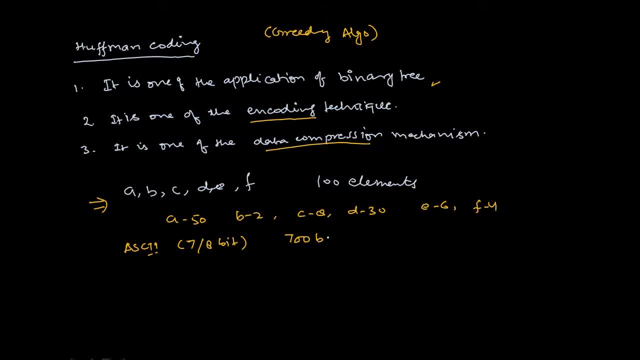 So it will require approximately 700 bits to encode one symbol. Now the point here is: if we use some 3 bit encoding, then the total number of bits required is 300 bits. And because 3 bits have a, you can assign the codes like if A is represented by 000, before B can be represented by 001. 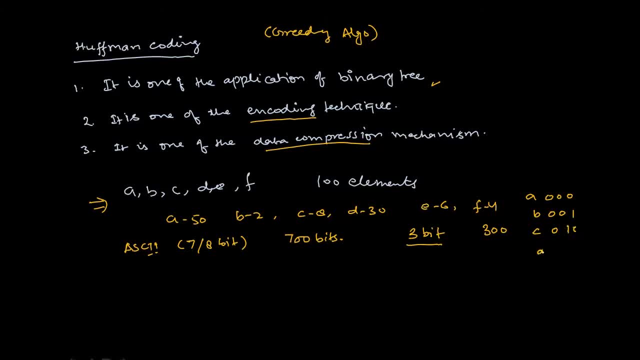 C by 002, C by 003, 0 1 0, D by 0 1 1, and E can be represented by 1 0 0 and F can be represented by 1 1 1. this is one of the way we can represent these symbols by 300 bits. 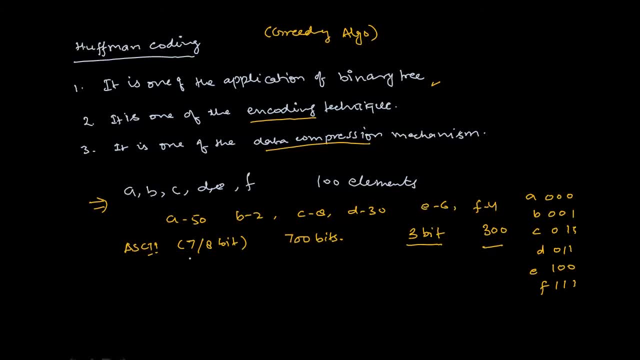 now, what is the idea behind the halfman coding? halfman coding does not represent each symbol by the same length of binary string. it assign the codes for each symbol depending upon the frequency of the symbol. so if the frequency of the symbol is high, then we will give it a less number of bit so that the string 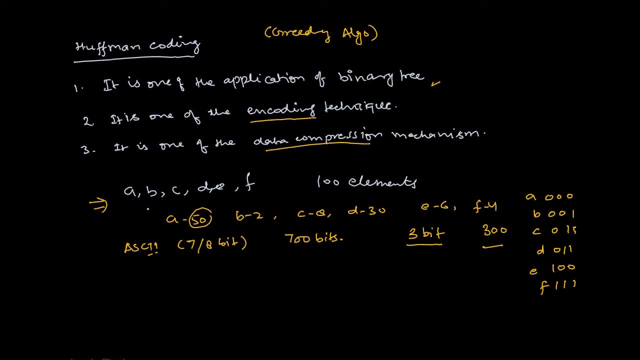 can be encoded into efficient bits or the less space. okay, so we construct a two-way binary tree in halfman coding and try to assign the bits or try to assign the codes according to their frequency. so for this example, if I generate a halfman code, so I start with the least frequencies. 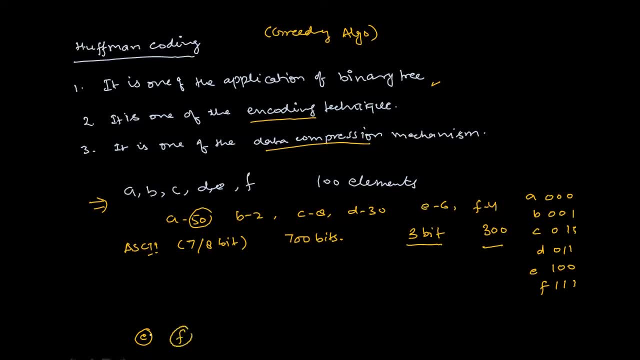 like E and F. I take two node with E and F, so E has frequency 6 and F has frequency 4. I combine these two, which is resultant intermediate node, tan. then this tan is inserted into the array. so okay. okay, let me again redraw it, because so to represent this example in: 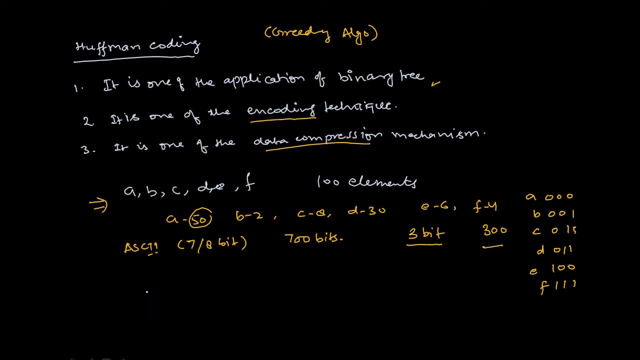 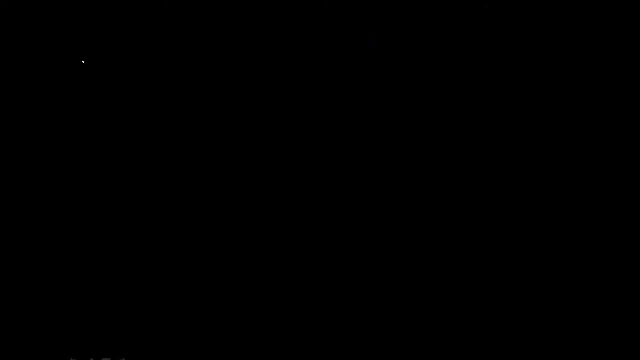 halfman coding. first you need to sort these symbols so according to their frequency, So B2, then F4, then E6, then C8, then D30 and A50.. Okay, now we construct a tree. So let me go to another page. Now I write the sorted sequence here. So we have symbol. 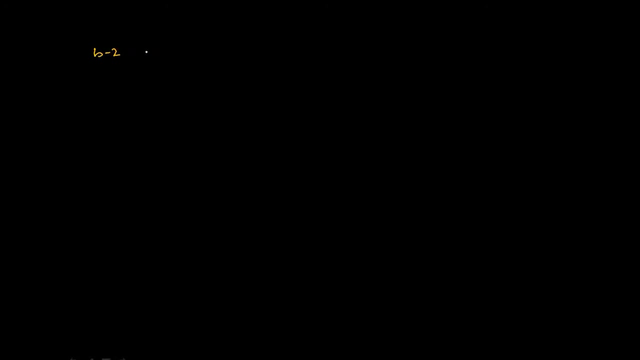 B with frequency 2, symbol F with frequency 4, symbol E with frequency 6 and symbol D with frequency 8,. symbol C- sorry, it is symbol E and symbol C with frequency 8, symbol D with frequency 30 and A with frequency 50. These are the symbols which is arranged in. 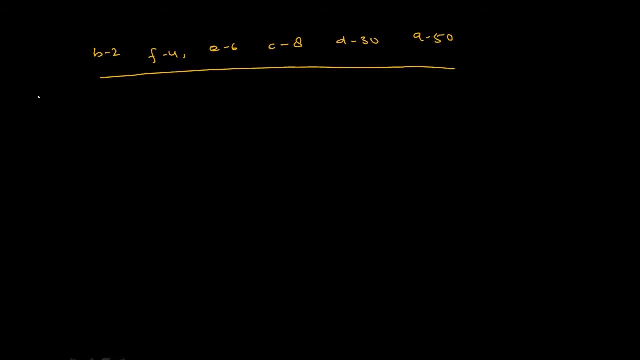 a sorted order of the frequency minimum to maximum. Now I pick any two minimum frequency, So I pick B and C And F. combine these two, it will result in an intermediate frequency 6.. I insert this 6 into my this sorted list. So 6 is inserted here and I combine the next element with this. 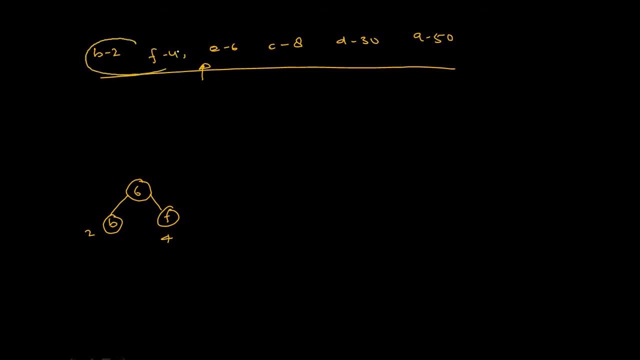 one. I remove these two, and so this 2 is replaced by 6 and 6 is inserted in the its right position in the array. Then 6,. next two elements are E and this intermediate frequency. So I write it here: E with frequency 6.. So this 6 and 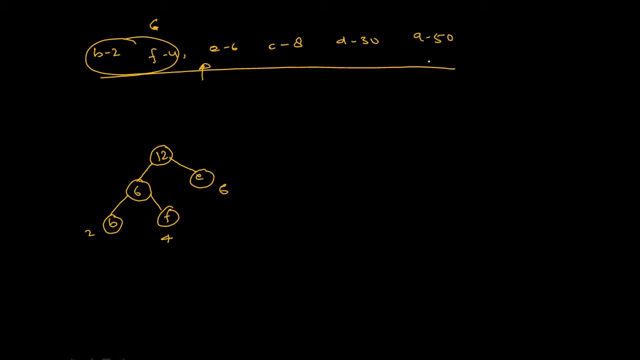 6 make value 12.. Then this 12 is inserted into the array. So 12 is inserted here. So then again I write the C here, Okay, And combine these two. So C has a frequency 8.. So the intermediate node has a frequency 20,. 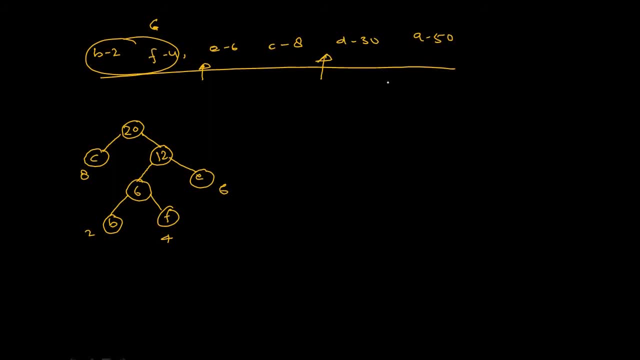 addition of these two. Then 20 is inserted at right place, So these two intermediate are replaced by 20.. And then we pick the next element, that is D, And D has a frequency 30. So this will result in intermediate frequency 50.. 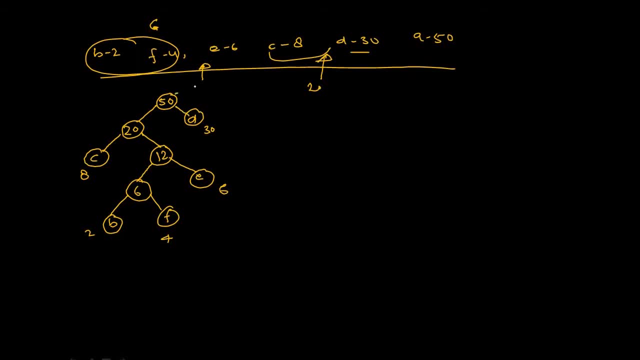 And then again we pick 50. Which is results in 100 frequency And this is A with the frequency 50. So we assign the code to the branches in the tree. So I have, I assign zero to the left branch and one to the right branch. 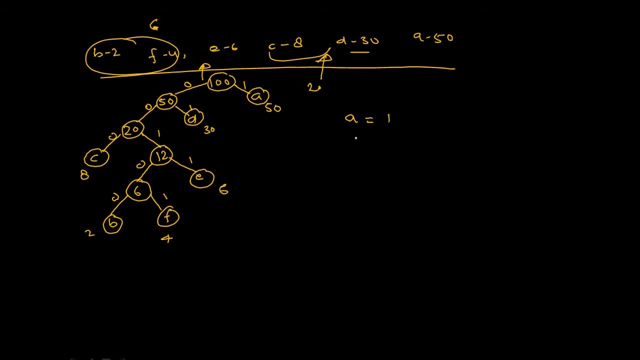 Now the code for A is one. Code for B is this: the path from root to B is 00100.. Code for C is 000.. Code for D is 01.. Code for E is 0011.. Code for F is 00101.. 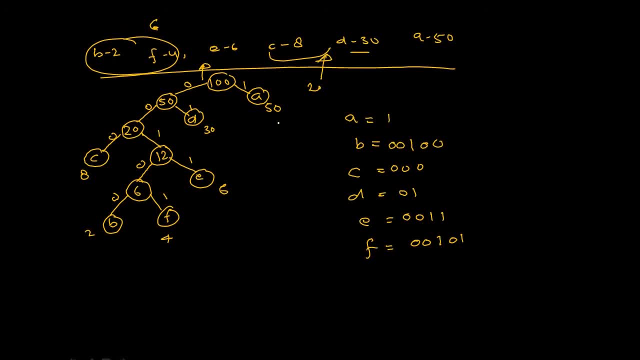 So you can see that node A have a highest frequency, So it is assigned a less code. Similarly, B have the least frequency, It is assigned a heavy code, So the total number of bits. So if I send this message by these codes, 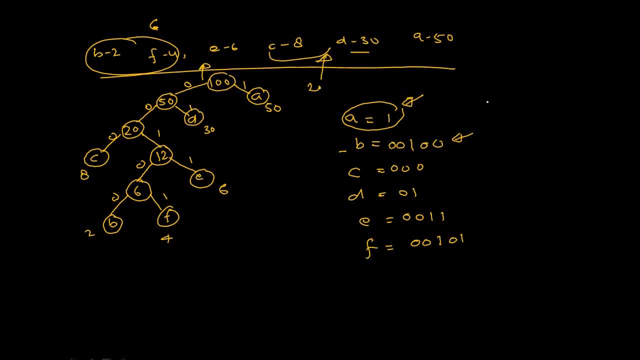 then because A is repeated 50 times, So the total bits required for is 50 into 1.. This B is repeated 2 times, So I can say that 5 into 2 times bits are required. Then this is repeated 8 times, So 8 into 3.. Then 2 into 30., Then 4 into 6.. And then 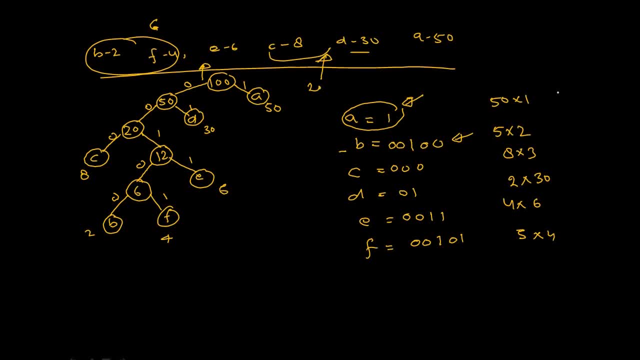 5 into 4.. So the total number of bits are 10.. Here it is 10. 24. Then, Sorry, It is 10. It is 24.. This is 60. This is 24.. 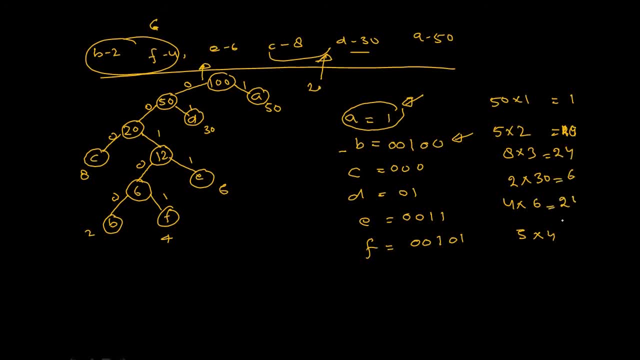 And this is 20.. Okay, Now, if we add these bits it will go to 8 bits. So if we encode the message using standard technique, like 3-bit encoding or 7-bit encoding, So these encoding will result in 300 symbols. So I can use at least 3 bits if I use a standard.